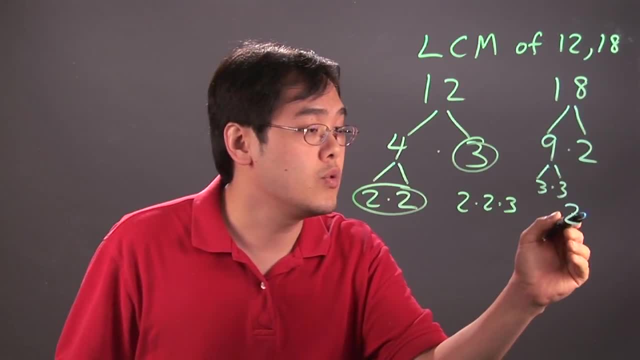 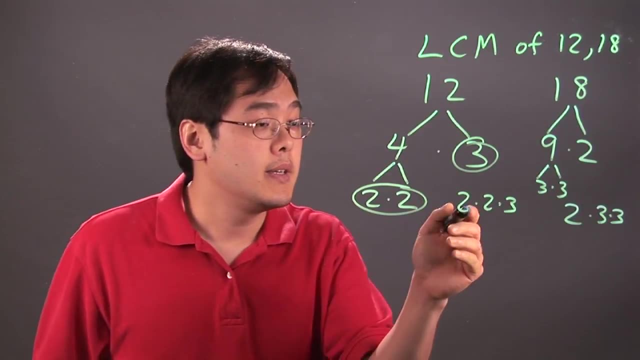 So 18 can be written in order 2 times, 3 times 3.. Now, when it comes to finding the least common multiple, what you want to think about is look at the number factors and see which number has the most of each number and circle it from there. So, for example, 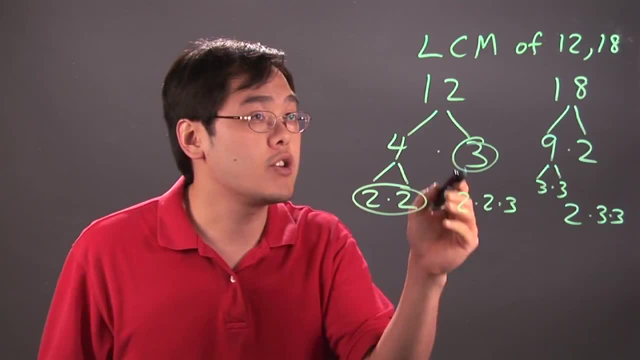 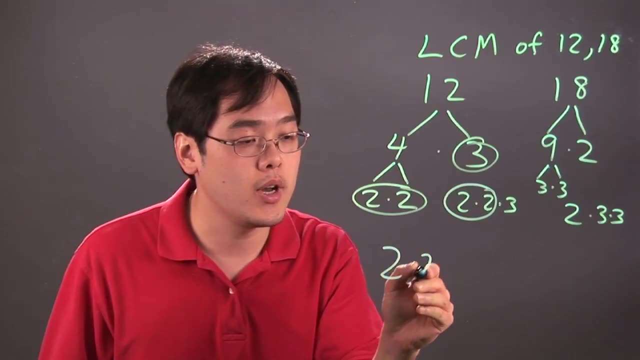 between 12 and 18, who has the most 2's? As you can tell, the 12 has more 2's and it's got two of them, So you're going to circle those two 2's. That's going to be part of your least common multiple. 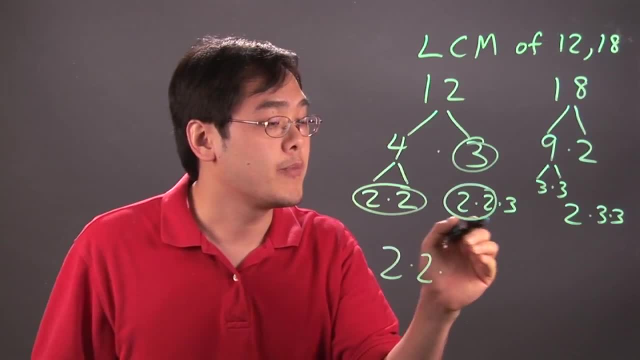 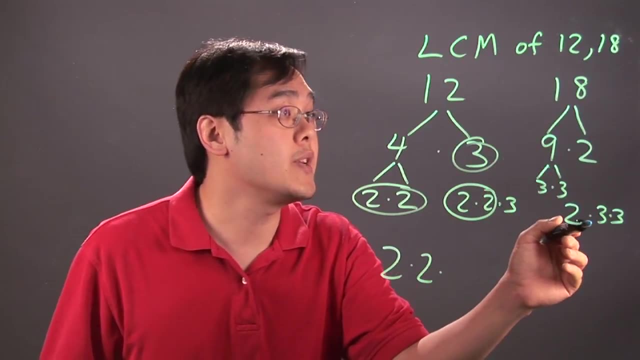 Next you move on to see if who has the most 3's and circle that amount. Now between the 12 and 18, the 18 has more 3's, so you're going to circle those two 3's Now if you ever have a tie. 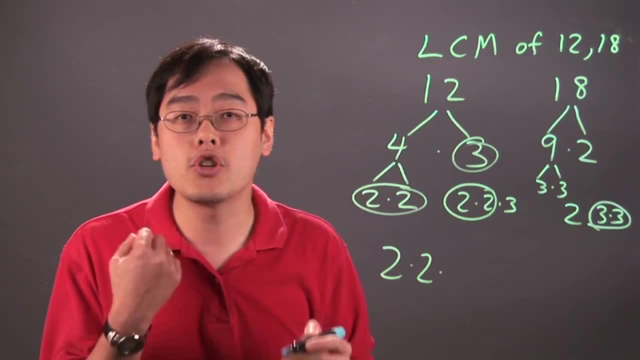 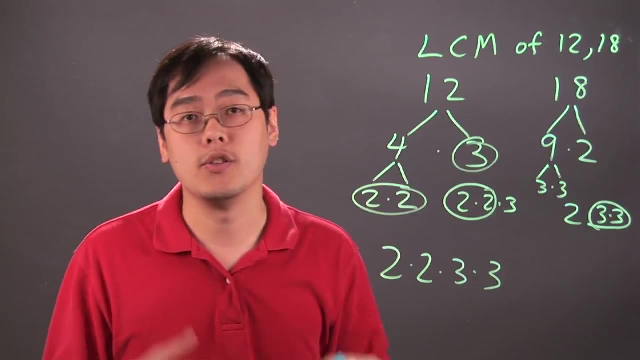 when it comes to LCM, for example, if both of them had two 3's, you just circle one pair, So the 3 and the 3 is part of the least common multiple, And then you multiply, Multiply what you have from here and that's going to be the LCM. 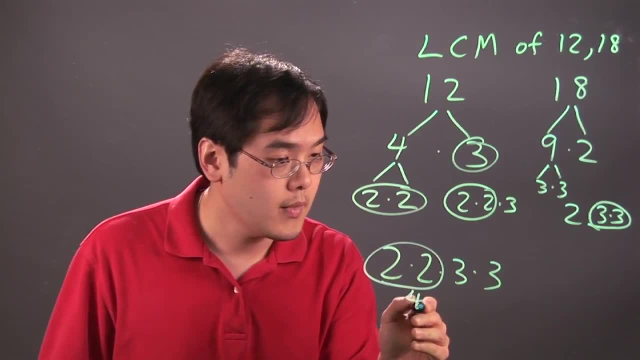 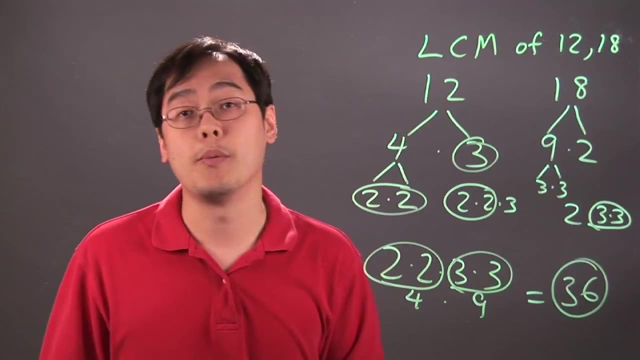 2 times 2 is 4.. 3 times 3 is 9.. And 4 times 9 is going to be 36, which is going to give you the least common multiple. So the bottom line is, when it comes to prime factorization, you break up each. 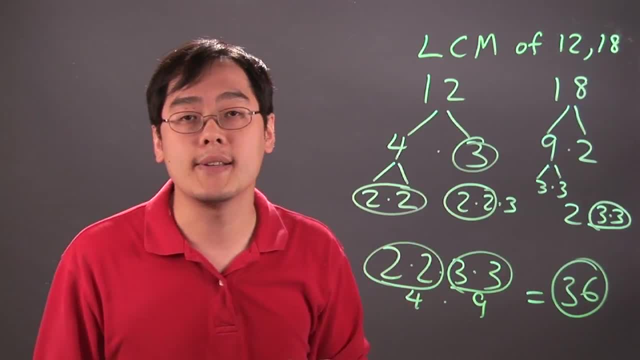 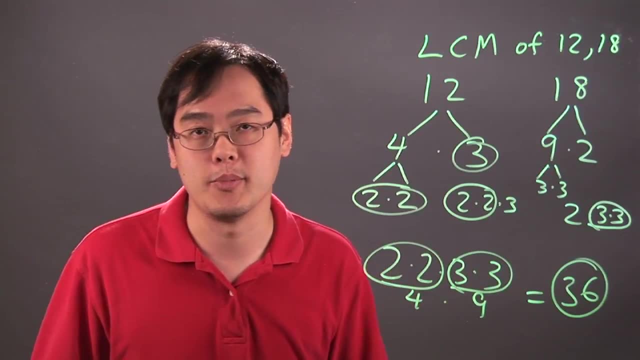 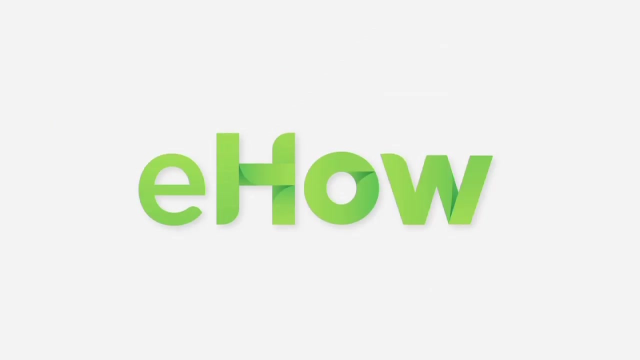 number as much as possible, and then you circle who has the most number of factors from each and you'll be good to go, And after you multiply them you'll have your least common multiple. So I'm Jimmy Chang. and that's how to find the least common multiple: using prime factorization. 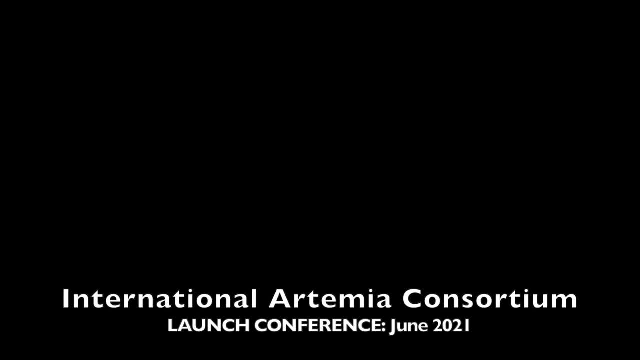 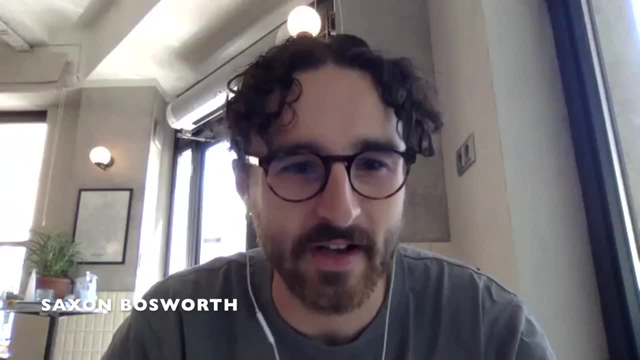 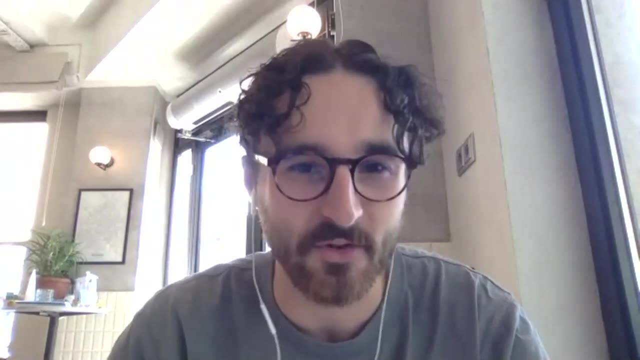 Hello everyone. it's a real honor and pleasure to be with you today and for Patrick to have kindly set up this meeting with you all. It really is a true pleasure- and to give you a little bit of backstory on myself. I think you know a little bit of information from the email, but I'm making a